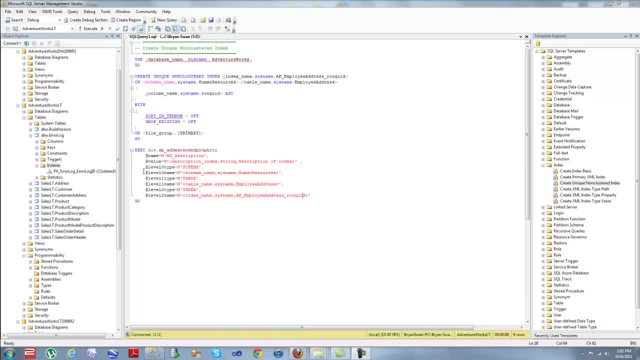 Okay, so let's talk about how you identify columns and tables. Now, this is just via the Template Explorer, okay, over here on the right right, And you guys can view this too. You just go up to View and then you hit Template Explorer, okay. 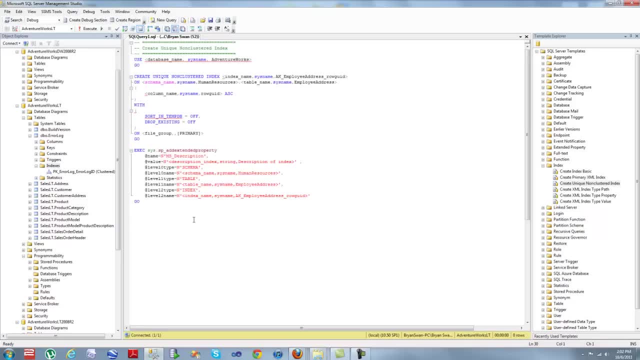 And this will give you a sample of what a script looks like to create an index. okay, But a much easier way if you want to create an index is simply to go down to your table, click Expand It. We have our columns. we have our keys. okay, 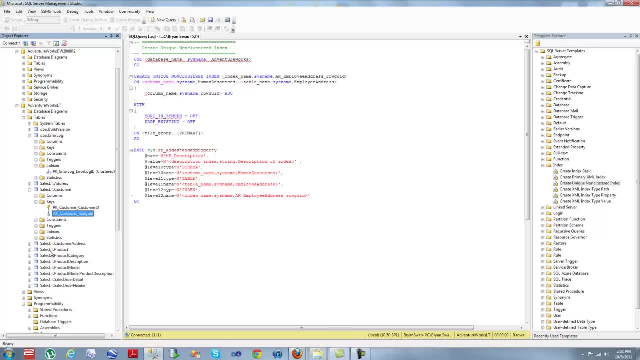 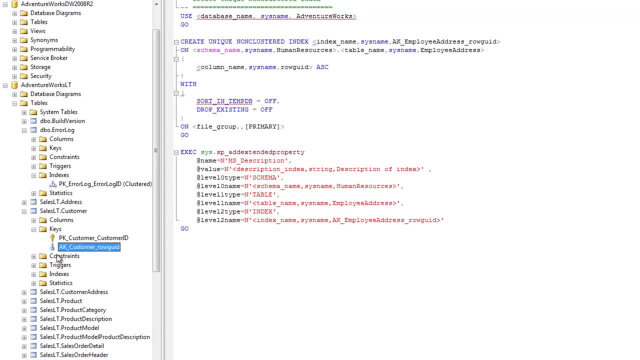 And this is, of course, a primary key, And this is an alternate key, I believe, And alternate keys, I think, are keys that are immediately available to be primary keys. Don't quote me on that, though, however, But let's scroll down to indices, okay. 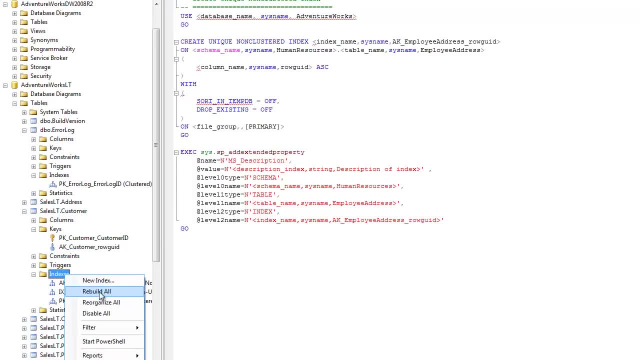 So let's right-click and we can put a new index. Now, why would we want to rebuild or reorganize all of our index or one of our indices? okay, We would want to do that when the index gets, when the table itself gets so fundamentally changed. 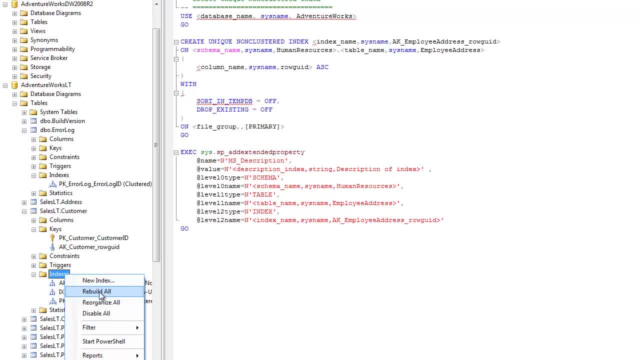 that the index that it's been originally created for doesn't necessarily directly correlate to that new data set, So it's not as effective. all right, Now you can create jobs in SSIS- very easy jobs, okay. that can have a nightly task to rebuild and reorganize all your indices, okay. 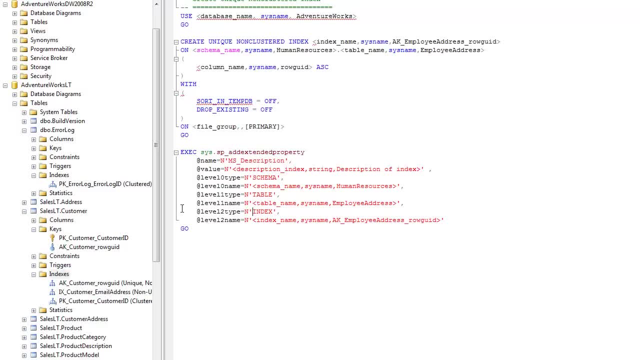 Now, when would it be a bad idea to make indices? In my opinion, and many others' opinion, the reason that you would not want to index certain columns is if you're constantly updating that table, it's going to take a lot more time to process updates. 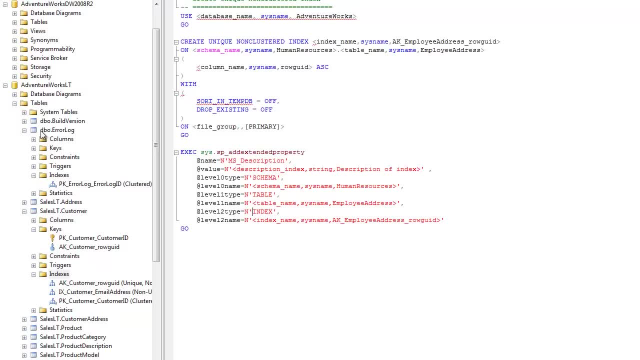 because those indices have to be affected again and your statistics may need to be calculated. So it's a good idea to have a new index and you can have a new index. that's not always going to be automatically calculated because of that, okay. 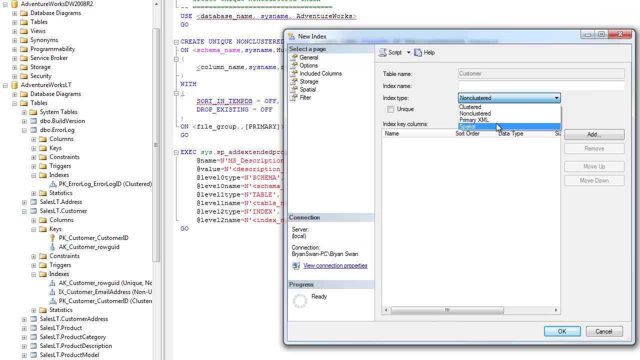 And that can be set up with this When I go to new index. all right, I have a choice between clustered, non-clustered, primary XML, which you're probably not going to use. spatial, which you're probably not going to use unless you're using. 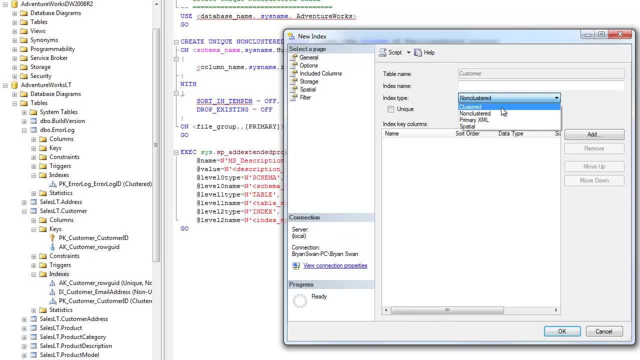 geographic data points and things like that. The bread and butter of indexing really is clustered or not clustered- okay, And you're only going to have clustered okay When someone asks you a question and some interviewer wants to be really smart and they say: 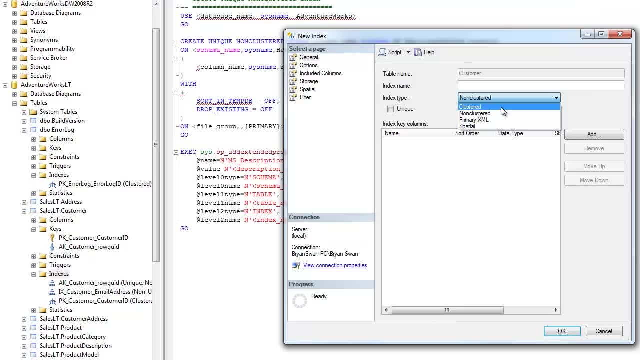 they should really. you can actually check them on this, because you can actually have two columns as a primary key. okay, It's a composite key, It's a composite clustered key and I can make that in the table if I go into table design. 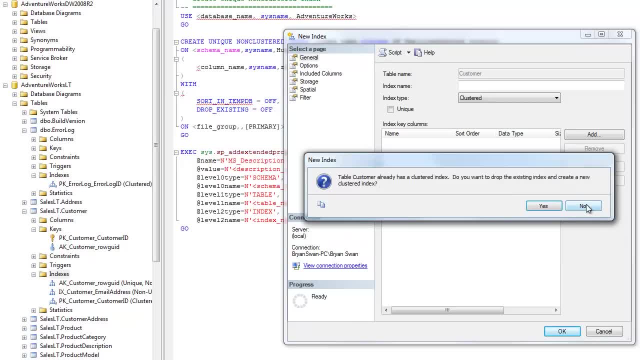 Now, if I want to go in and make this index, let's not make clustered, let's just make a non-clustered one, because I think there's already one out here. Now, do we want to make that unique? Well, is all the data unique? 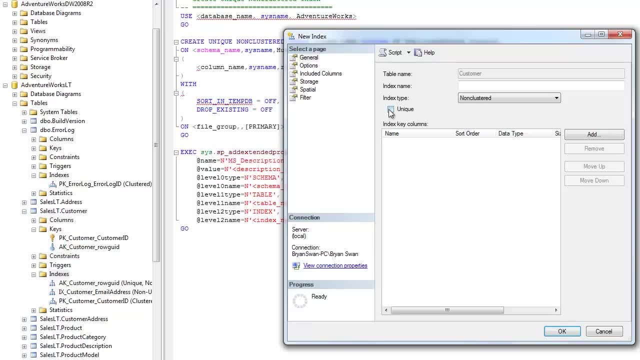 If it is, then let's make it. If not, if it's Mary Joe, Jill and Bob, then that can be unique. If it's Mary, Mary Joe, Jill and Bob, obviously that can't be unique because there's duplicates in there, okay. 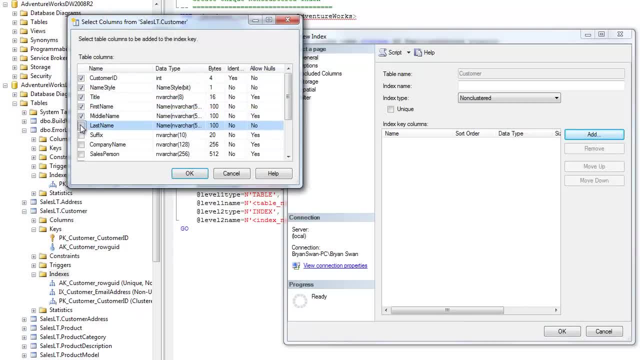 So let's just add this and we can choose what we want to include. So right now we are making a composite index. Why? Because we're including more than one column in this index. okay, I'm going to go ahead. oh, I need to enter a name. sorry, blah, blah, blah, okay. 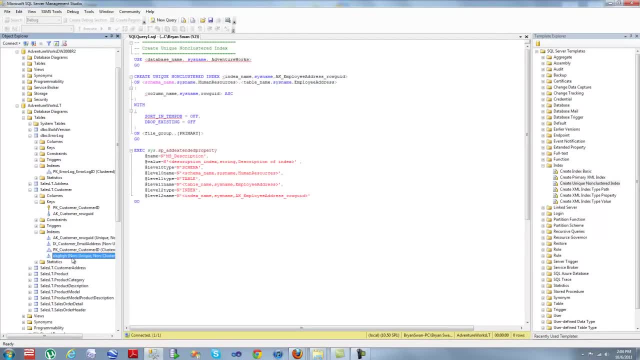 Put it in there. executing: that is created. As you can see, this is now created. If I want to drop this index, I can. If I want to disable it, I can. If I want to rebuild or reorganize it, I can. okay. 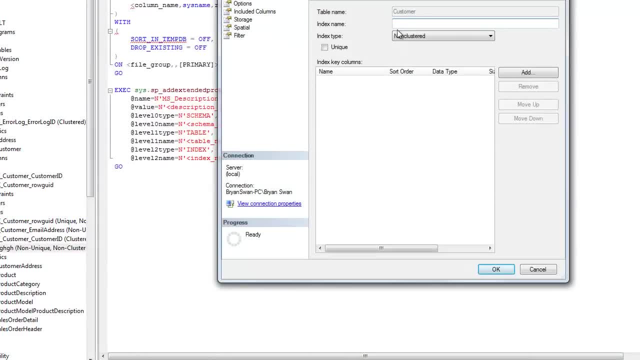 And you saw if I want to do a new one. you see, under options, it automatically recomputes the statistics based on it. However, you need to create statistics on it if they're going to get recomputed. okay, We can talk about that later. 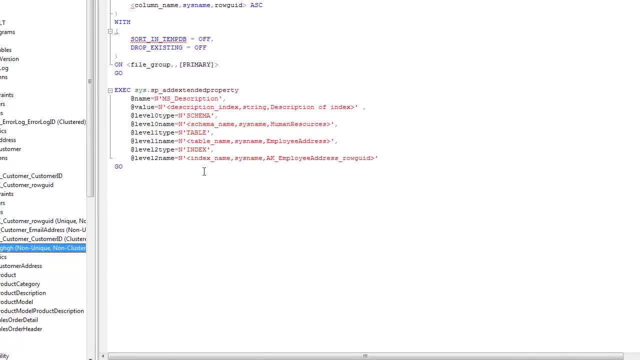 Just go ahead and Google that. if you want to talk about creating statistics, That's more associated with the Database Engine Tuning Advisor, okay, So you know, you run the SQL Profiler, You export it to a table, Then you push that either via the table that you've exported it to or via the script. 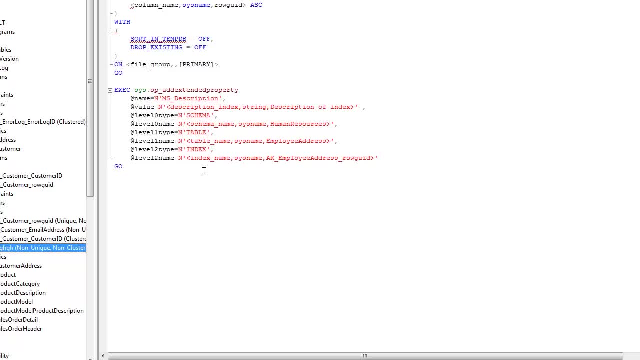 Push that into the Database Tuning Engine Advisor, which is an incredible tool, And it will tell you if you need to create statistics. if it doesn't like the index you've created, if you could use an index there, And it writes the script for you. 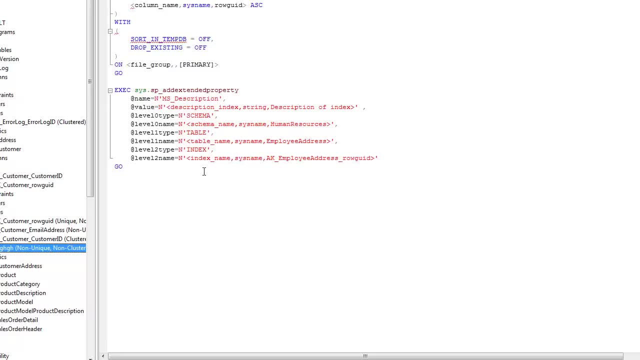 It's one of the most incredible tools ever, okay, Right now I'm on my home PC with Express and I don't have access to that. okay, But you know it's the best tool as far as entirely of SQL Server. 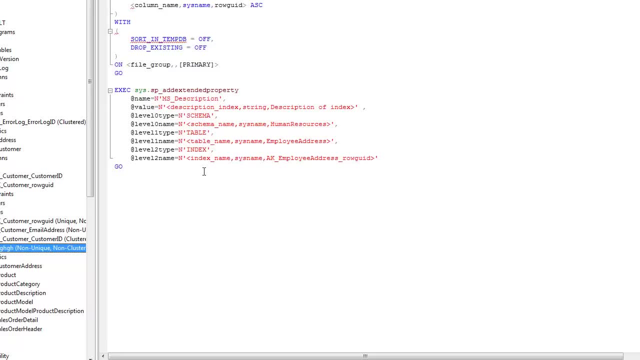 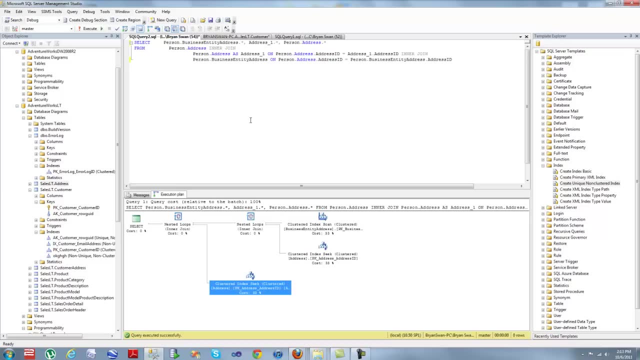 Okay, So let's migrate over to. Okay. so now let's talk a little bit about how we find what tables need to be indexed and what tables don't. This is all sans using the SQL Profiler and putting that information based on the activity, because the SQL Profiler tags basically every piece of activity that your database is facing and encountering. 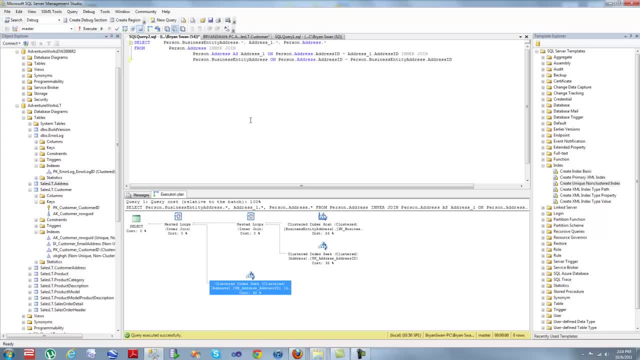 And it records it. And then when you place that data into the Database Tuning Advisor, it churns out. It records all the recommendations based on that and the structure and design of your database. okay, So this is just within a normal query, all right. 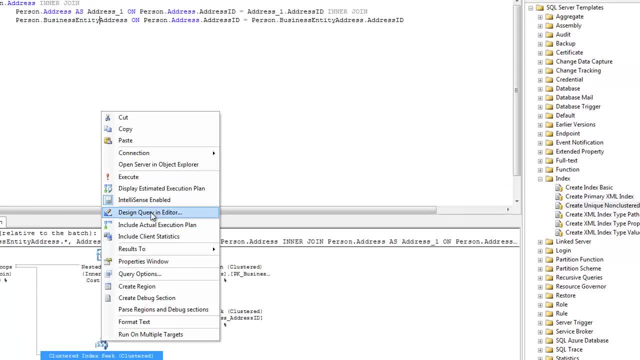 So I just went into Query Designer. I just took a bunch of tables in and linked them together. okay, Now I'm going to right-click again and I'm going to include the actual execution plan. okay, Now, when I click on that, this pops up: okay. 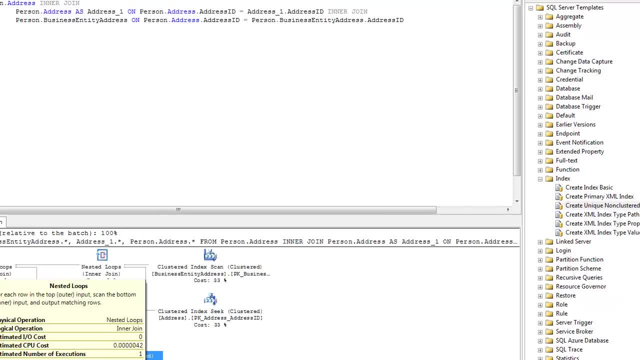 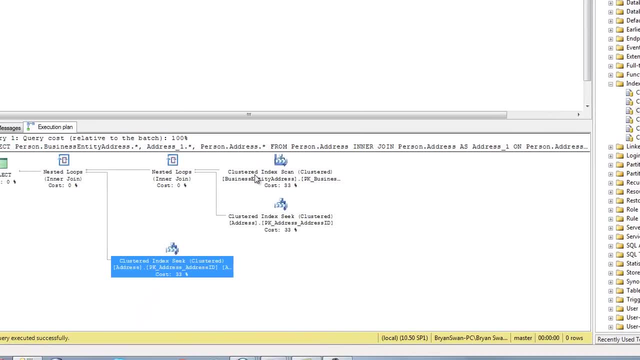 So what is good and what is bad within here? okay, So index seeks are the best. okay, That means what you're doing is extremely well done. This is well designed, okay. Index scans are not the greatest, but they're still better than table scans, which are basically the worst. okay. 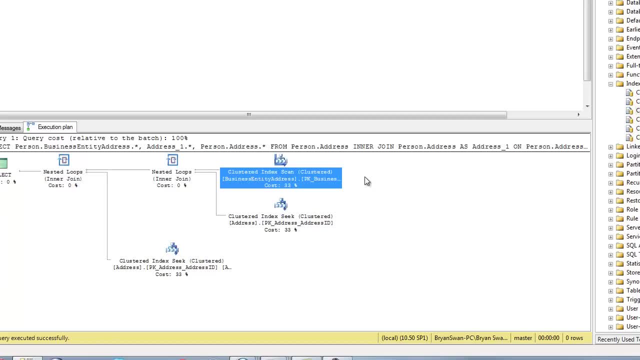 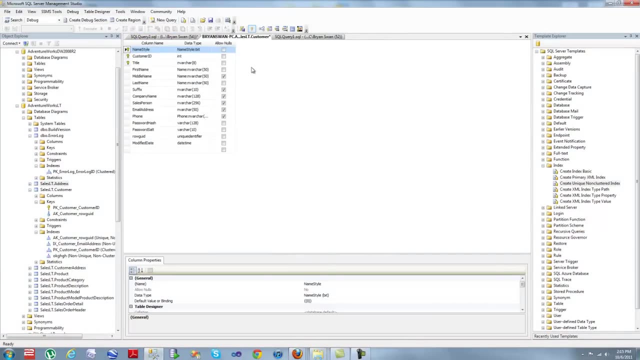 That indicates that there's no indexing of any real design within your query, ie the tables themselves. okay, Because these all represent basically tables and joints. okay, Now we can go over into. This is going back to the question that I posed about the multiple priors. 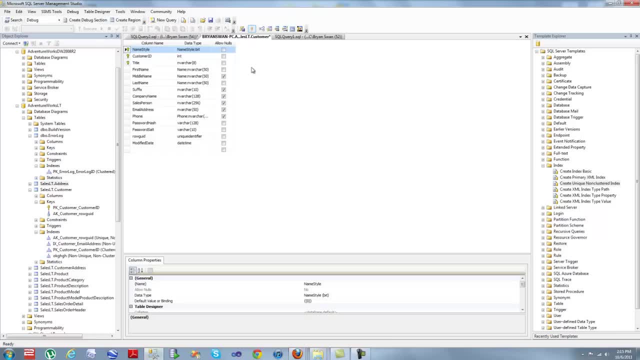 Okay, So you can have 10 primary keys, so to speak. okay, Now, of course, you can only have one primary key, but you can have one primary key that encompasses several columns. So, essentially, I mean, it's within a possibility to have, you know, a 10-column primary key. okay. 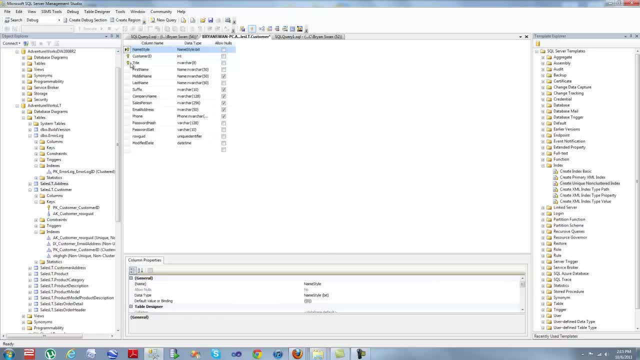 All you do here is you simply just highlight, You just shift-highlight, and then you hit the key button. okay. Now, if you wanted to really look at it, you just go to indexes and keys. okay, And these are the different ones. 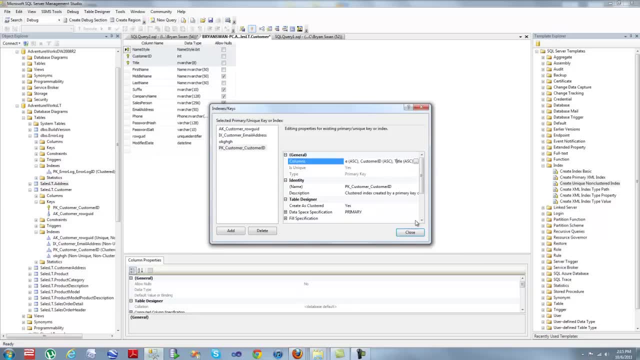 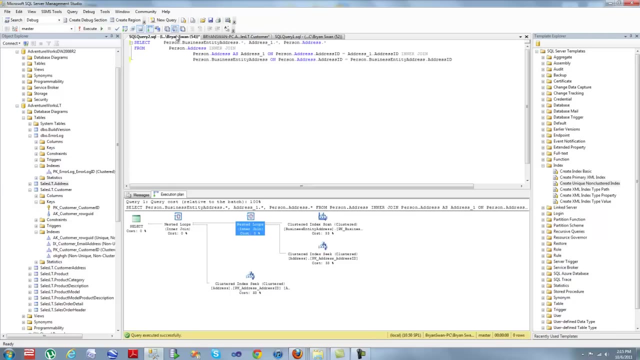 And, as you can see, here we have three columns included. okay, So now this is a composite of primary cluster, clustered index or composite primary key. okay, And let's move now onto. Okay. so now I just pulled in another query and I pulled in the actual result set. 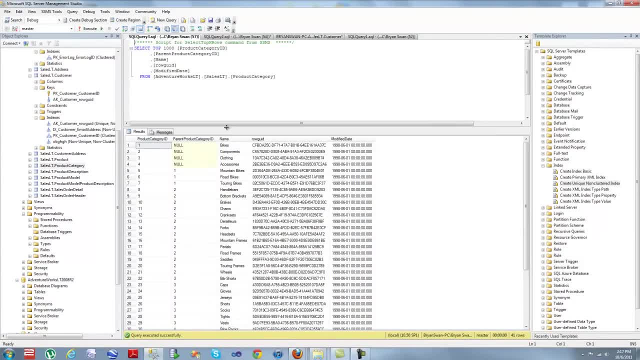 Now, the final point I want to make is on the decision-making process of how to optimize. Okay. so let's say we want to update a column, okay. So why do we want to update a column and put an index on it? okay? 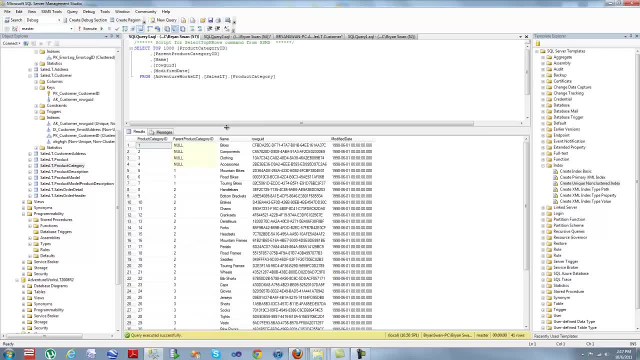 What are the best columns to use? okay, We want data that is very multifaceted. okay, Think Social Security numbers, Think product IDs, Think serial numbers. okay, Those are the best types of columns to slap those indexes on. okay, 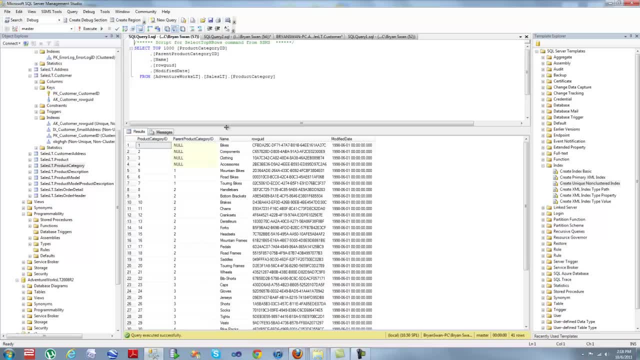 And you will see a large increase in your speed from this. okay, So definitely take a look at the Database Engine Tuning Advisor. It's incredible. It comes stock with SQL Server, okay, as does all the business intelligence add-ons. okay. 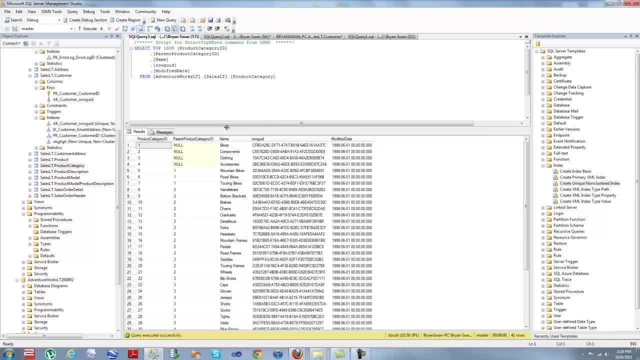 And you know, for the same platform in Oracle or whatever you know, Oracle costs $5,000 per processor for their version of the Database Engine Tuning Advisor. okay, SQL Server is just as good and one-fourth of the price, and it's incredible.